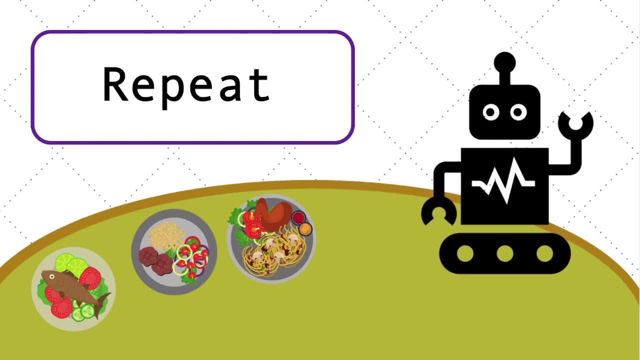 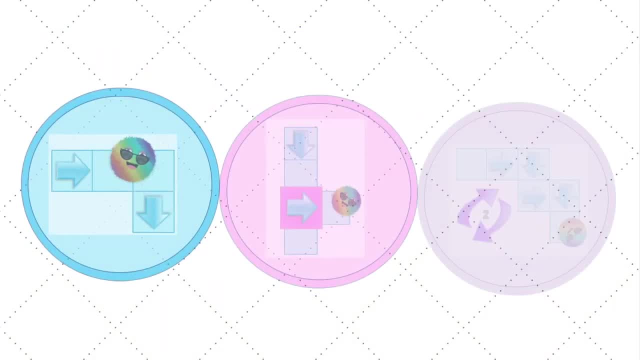 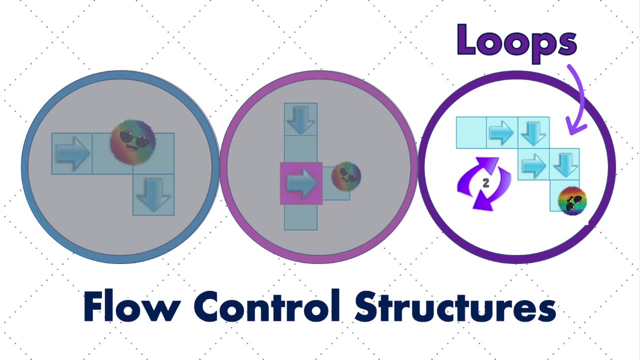 way to tell a computer to repeat an action without needing to repeat all the code. This command is called a loop. In programming, loops are the third of the flow control structures and allow us to use just one command to repeat the same process multiple times and complete a task. Loops are all about keeping your 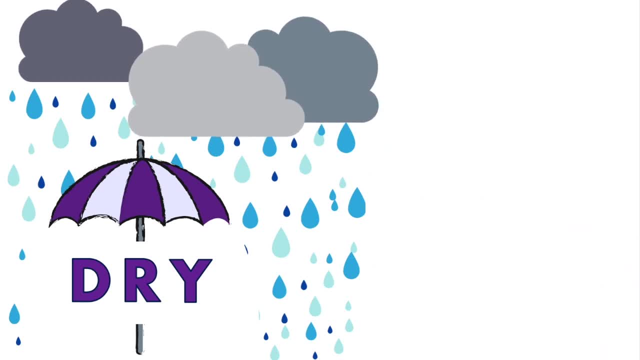 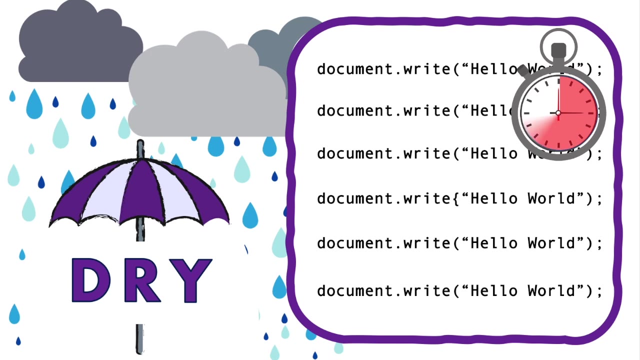 code dry. Dry means don't repeat yourself. So what's the problem with repetition? Well, typing out the same code over and over increases programming time. Also, if you have to write the same thing again and again, you're more likely to make a 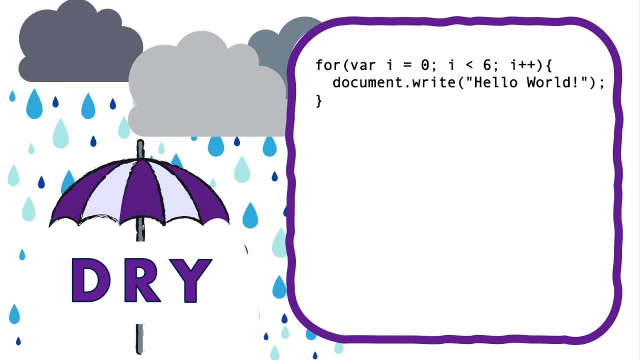 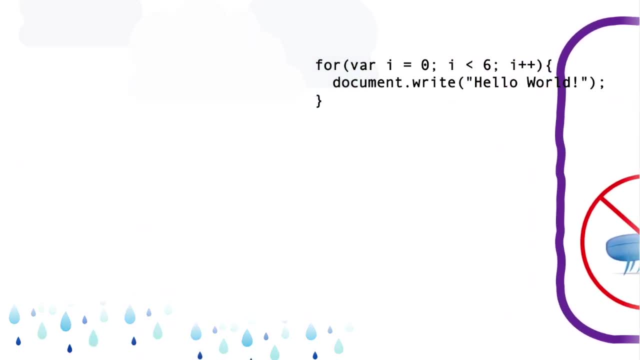 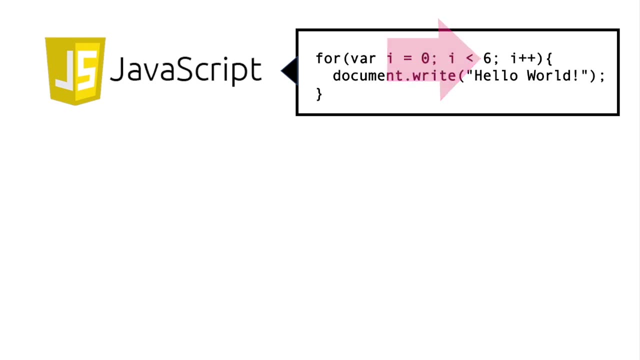 mistake somewhere, Make your code repeat, Make your code shorter with a loop. Now it's easier to debug and saved you time. So what does a loop look like in a program? Well, in JavaScript, loops look like this: This code will loop six times, But in Codable this is what we use to. 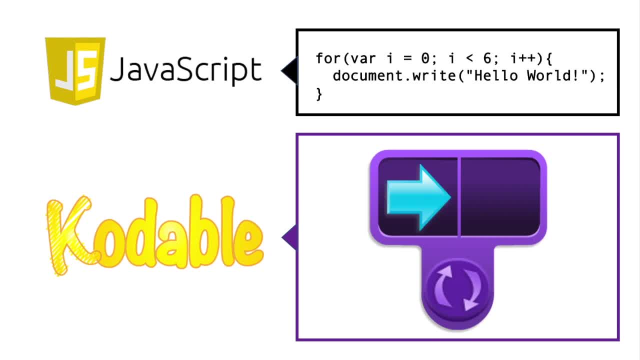 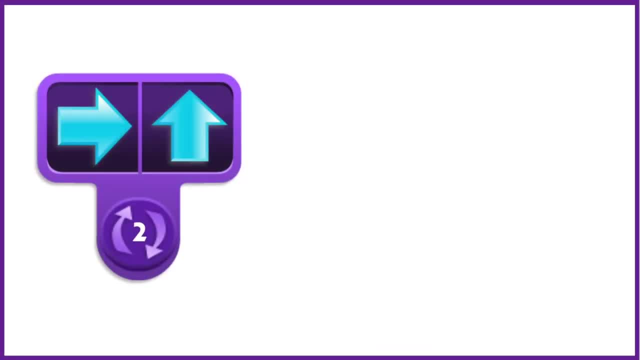 program a loop. This looper will repeat two commands a certain number of times to achieve an outcome. A block of code like this works. the same as code in class, code like this In both. your fuzz will move right up, right up, But what do? 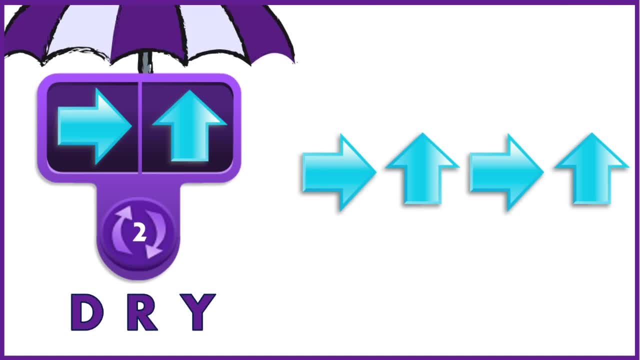 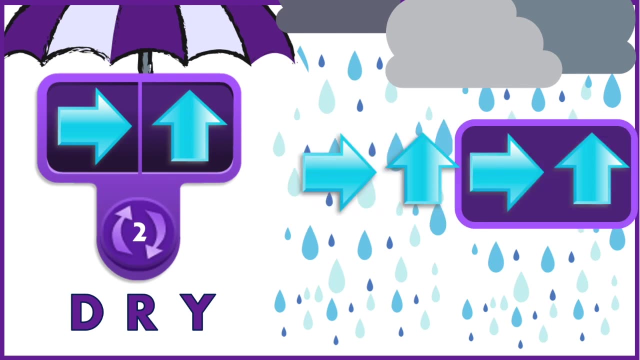 you notice about the two programs. This first option is shorter and drier. It will only take up one command bin in the game. The second option is not dry at all. It uses four commands and repeats the same commands twice. Now it's your turn. Use other commands. Use the same commands, but repeat them. 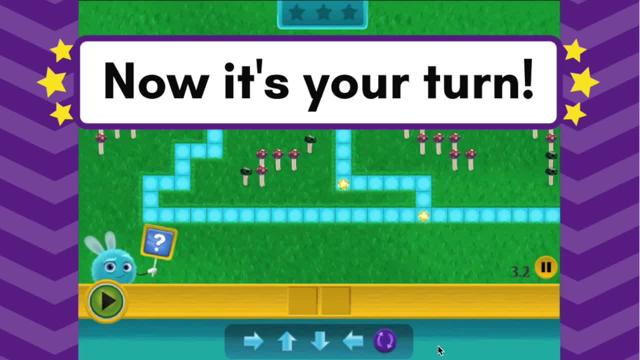 twice. Not the same ones over and over. Not the same ones over and over over. Not the same ones over and over. Not the same ones over and over. Not the same ones over and over. few commands as possible to get the fuzz through the maze. Start by looking at the 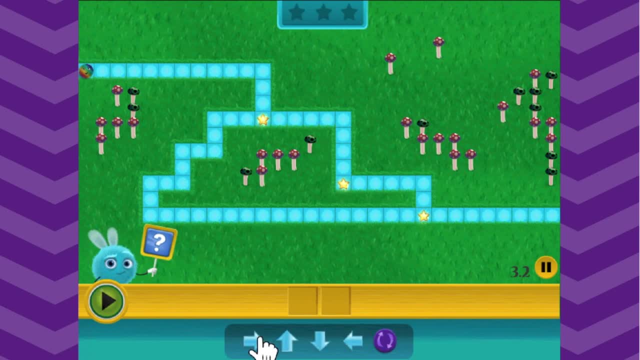 maze for patterns Here. I want my fuzz to move right and then down, right, down right, down right. Instead of dragging out all those repeating commands, I can use the looper and set it to loop the commands down and right three times.